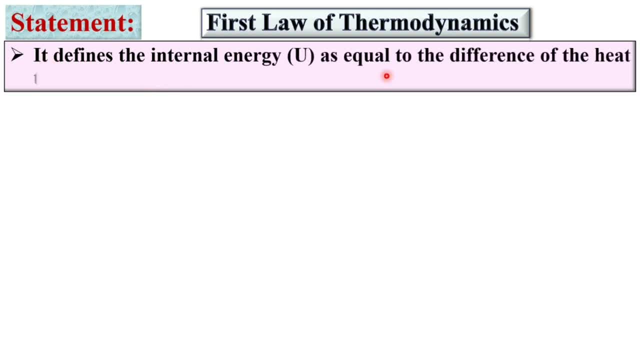 it is like that It defines the internal energy U as equal to the difference of the heat transfer Q into a system and the work done by the system. So I can say, when a system undergoes change of state, both heat and work transfer takes. 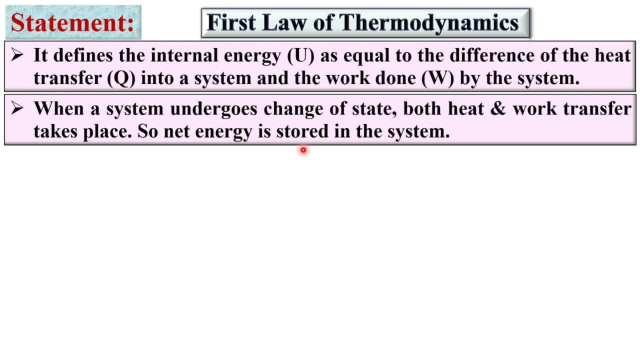 place. So need energy stored in the system. so we can say Delta E. that means the net energy stored. that is equal to Q minus W, and here we have written that energy that is equal to the difference of the heat transfer Q into a system and the work done by the system. 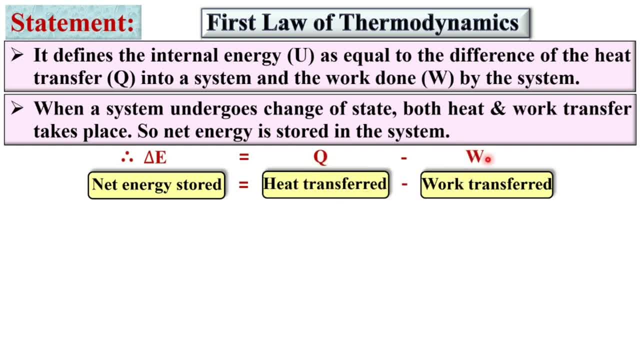 so here, Q is the heat transferred and W is the work transfer and the difference of these two, that will be the net energy stored into the system. so let's try to understand the same statement with the help of this figure. so let's consider: this is the one system and that is the state 1, if you supply. 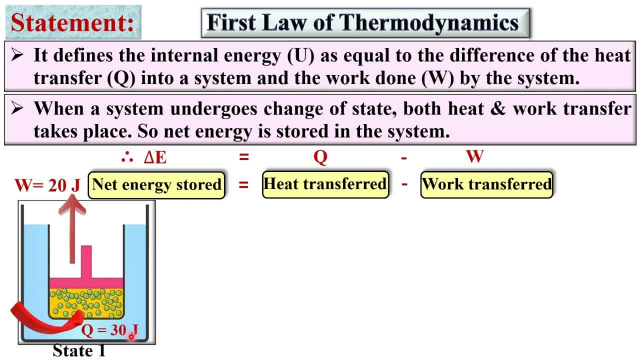 some of the heat Q and that say, for example, 30 joule, then this system will expand and so that there will be some output at the piston end and that work done. say for example, 20 joule, And this is the state 2. here you can say: due to the heat supply, the system will expand. 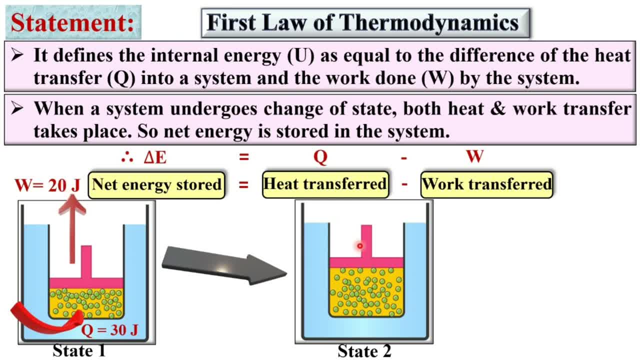 and so that you will get the output work done over here. So this is the state 1 before supplying the heat and this is the state 2 after supplying heat. So we can say, as per this equation, delta E, that means the change of energy during the 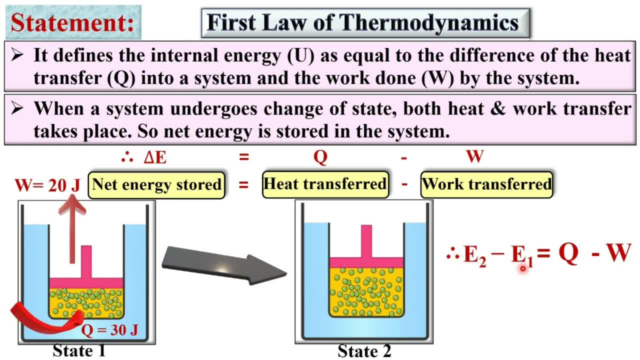 process 1 to 2, that is E2-E1 is equal to Q-W. So here you can say E2-E1, that means change of energy and Q. here you can see that is 30 joule minus W is equal to 20 joule. 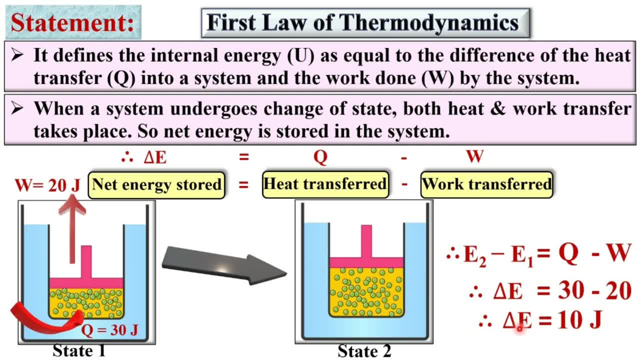 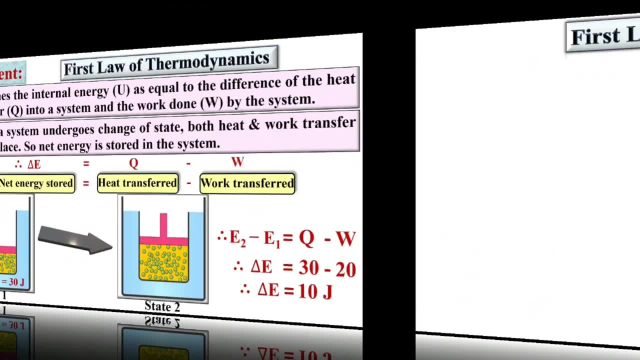 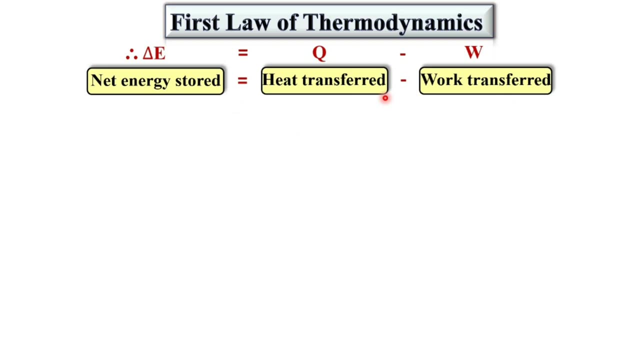 So you will get: delta E is equal to 10 joule, So that energy that is stored into the system. So now I think you can understand the statement of the first law of thermodynamics with the help of this example. Now already we have discussed this is the mathematic equation of the first law of thermodynamics. 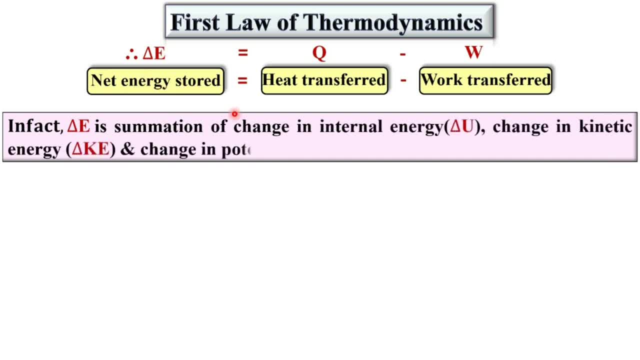 In fact delta E- that means net energy stored- is actually the summation of change in internal energy, change in kinetic energy and a change in potential energy. So we can say in mathematical way: delta E That means the stored energy. that is always equal to change in internal energy plus change. 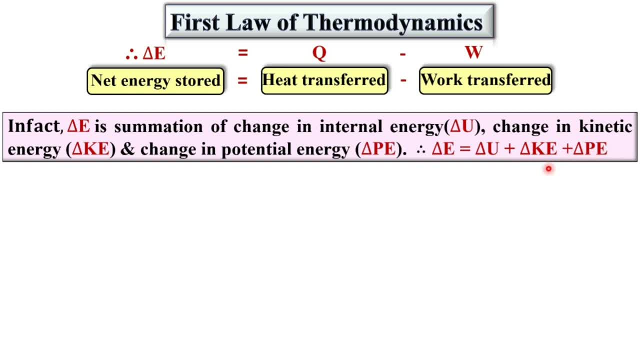 in kinetic energy plus change in potential energy. But for a closed system mass is fixed. you know that. So there is no elevation, that means change in potential energy is equal to zero, and no movement, that means change in kinetic energy is equal to zero. So if I consider from this equation delta KE and delta PE, both are zero, so that delta E 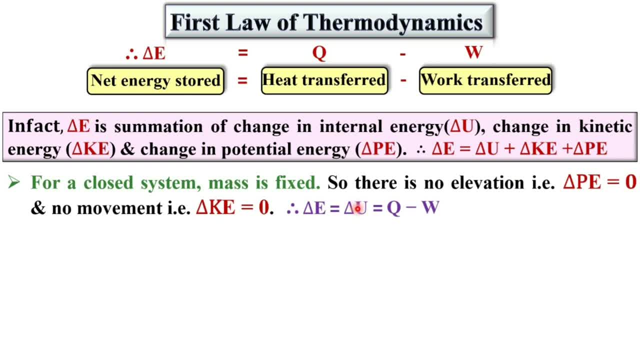 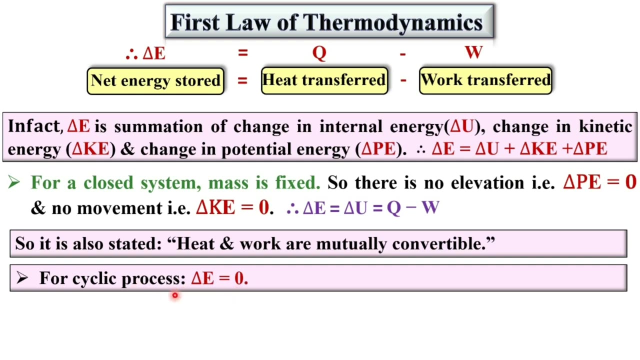 is equal to delta U. Now also you know that delta E is equal to Q minus W. so I can say: delta E is equal to delta U is equal to Q minus W. So from this equation you can say: heat and work are mutually convertible. If you consider for a cyclic process, then once again you know that. 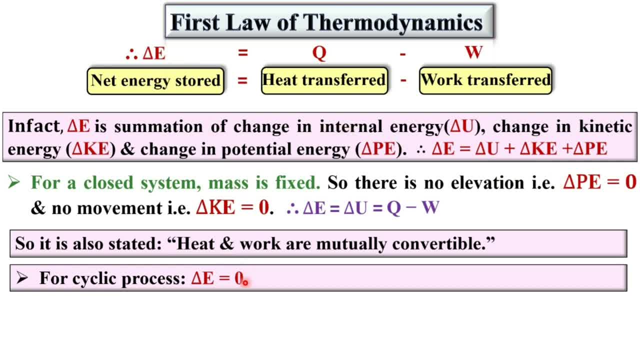 change in energy is equal to zero because of for the cyclic process, the system again returns to its initial state and so that there will be no any energy stored into the system. So you can say delta E is equal to zero. So from this equation, if I put over here a, delta E is equal to zero. so I can say Q is. 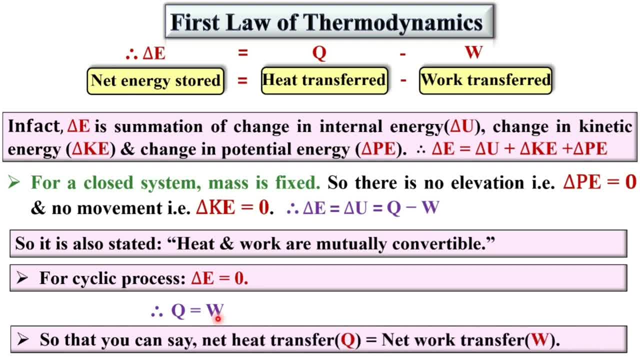 equal to W, So that you can say net heat transfer Q is equal to net work transfer. So this is the very simple mathematical form of the first-lobe thermodynamics. Now the application of the first-lobe thermodynamics. Now the application of the first-lobe thermodynamics. 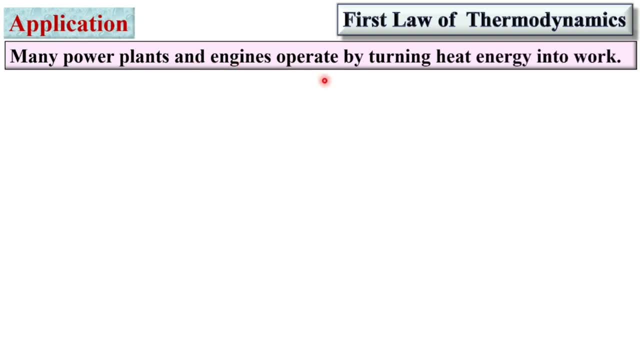 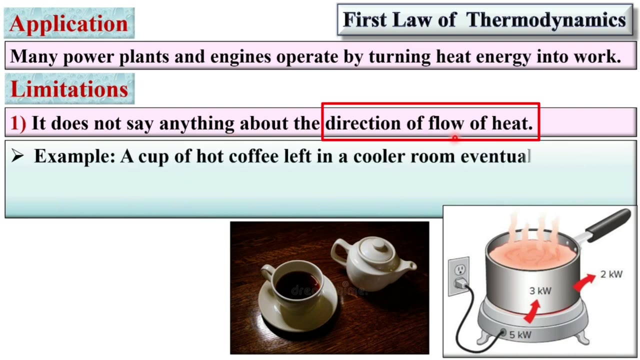 So many power plants and engines operate by turning heat energy into work. Next limitations: It does not say anything about the direction of the flow of heat. So very important first-lobe thermodynamics does not say anything about the direction of flow of heat. Example: a cup of hot coffee. 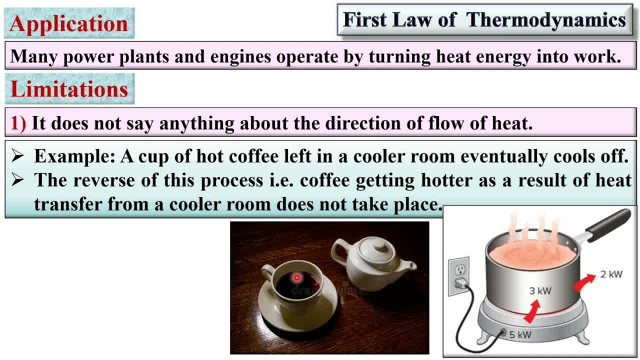 left in a cooler room eventually cools off. Very simple, you can understand. but now the reverse of this process- that means coffee getting hotter as a result of heat transfer from the cooler room- does not take place. So this low does not say anything about the direction of the flow of heat. That means the heat will flow from the coffee. 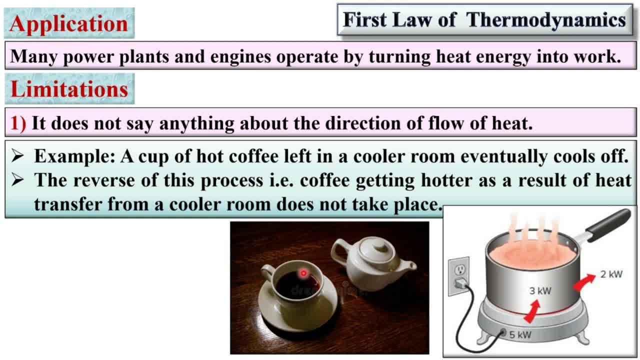 to the room or from the room to the coffee. Next, practically it is not possible to convert the heat energy into an equivalent amount of work Because of previously we have seen that the Q is equal to W, but practically it is not possible to convert the heat energy into the equivalent amount of the. 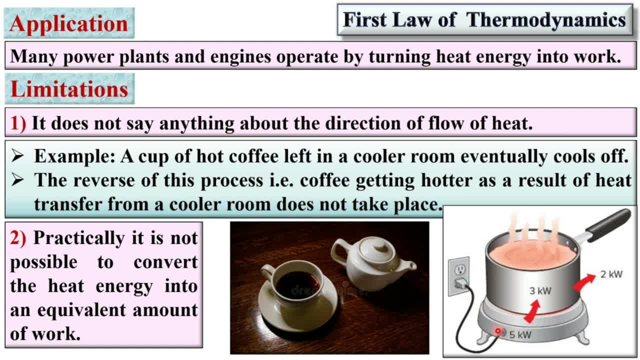 work. Let's see over here: if you supply some of the heat energy to the coffee, then the heat energy will be converted into the equivalent amount of the amount of input as five kilowatts, and that is in the form of heat energy. So only some of the portion will be converted into the work done and the remaining amount will be lost into the system. 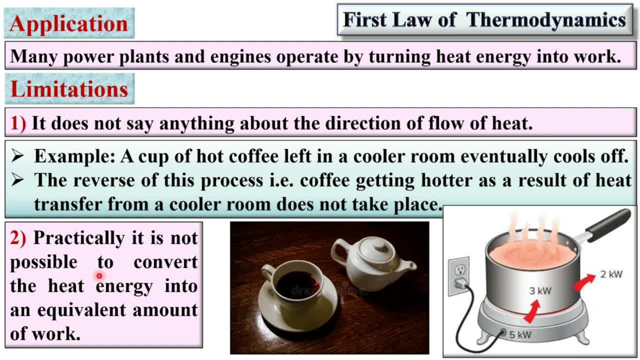 So always there is a loss in the system, So you can't convert completely the heat energy into the equivalent amount of work. So put your valuable feedback on the comment box for motivating me to make more videos. Thanks, my dear friends, for watching this video.